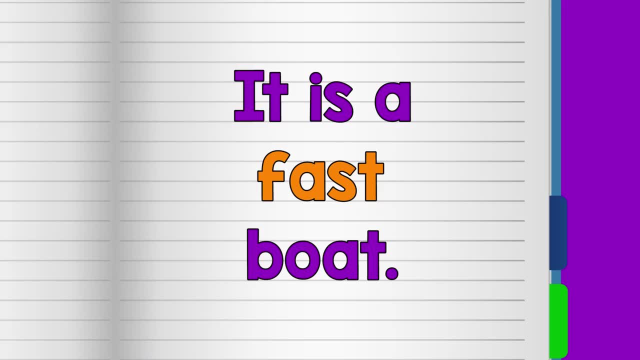 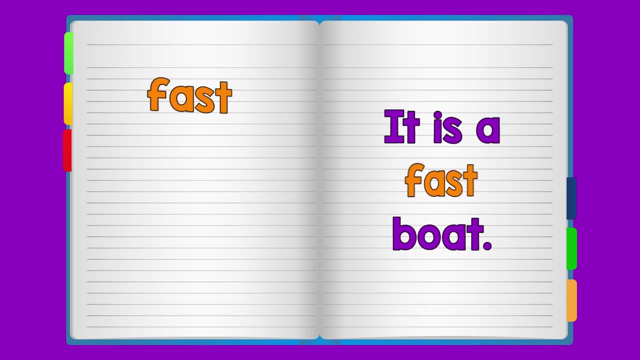 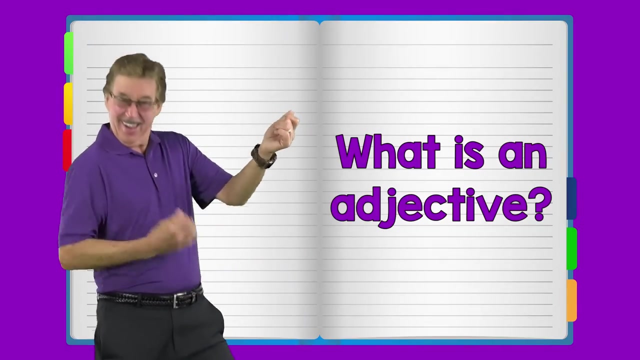 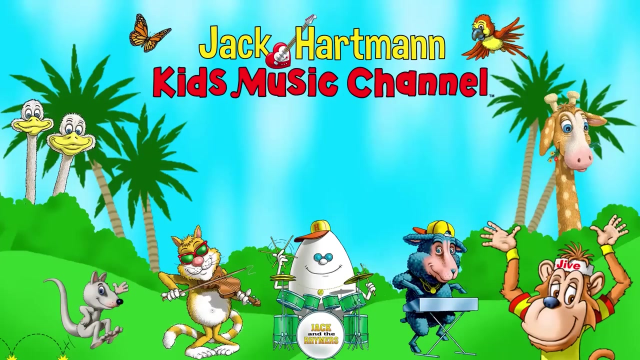 It is a fast boat. It is a fishing boat. It is a wooden boat. It is a whale boat. Fast fishing, wooden whale are all adjectives that describe the boat. What is an adjective? What is an adjective? Fast fishing, wooden whale are all adjectives that describe the boat. 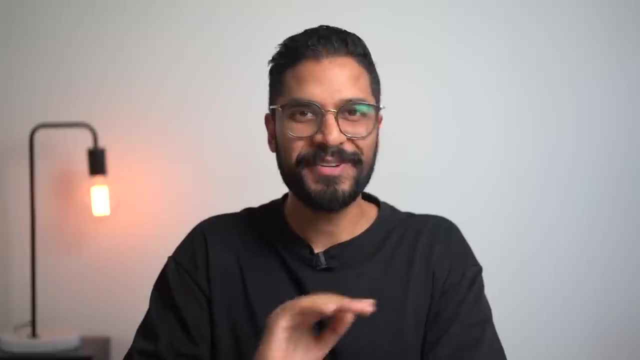 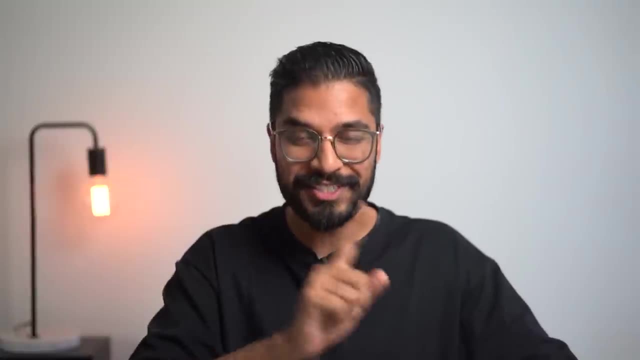 Oh, who doesn't like a good prediction video? In this video, I'm going to share with you exactly what I think is going to happen to property prices in Australia over 2023,, 2024 and beyond. If you're interested, definitely keep watching. 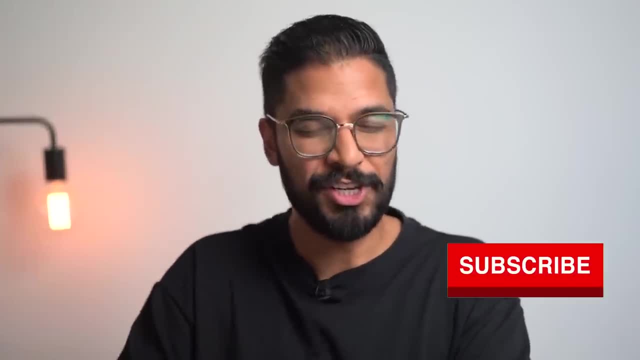 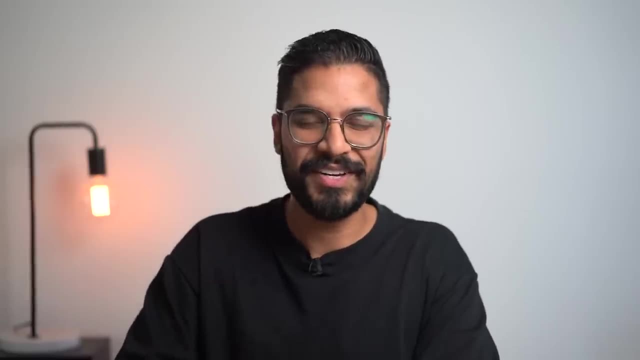 Hey guys, my name is Ravi and welcome back to Personal Finance with Ravi Sharma. If you're new here, smash that subscribe button, because I talk about real estate, cryptocurrency and financial freedom. Now, before you jump into the real nitty gritty of this video, I've got to let 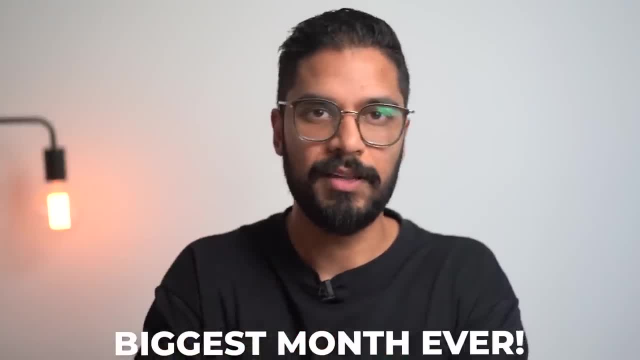 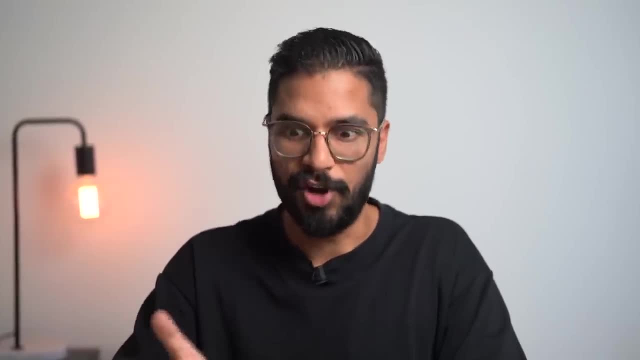 you know, we've just recorded our biggest month ever when it comes to the buyer's agency, So I'm very thankful, very grateful, that you guys are in a position to start making moves. I think a mass majority of people are going to move in 9 to 12 months If you guys are here and you're 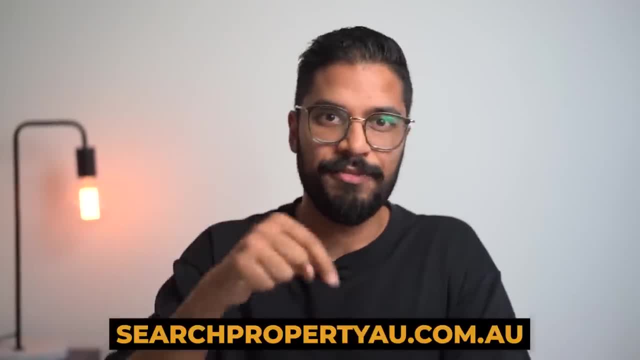 making those moves. that's fantastic. If you're interested in joining the buyer's agency, definitely go and click the links in the description below, or you'll find my email in the pinned comments. Now, with these price predictions, I'm going to look at three graphs. 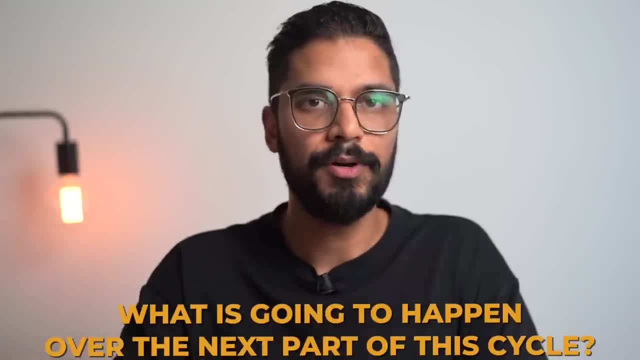 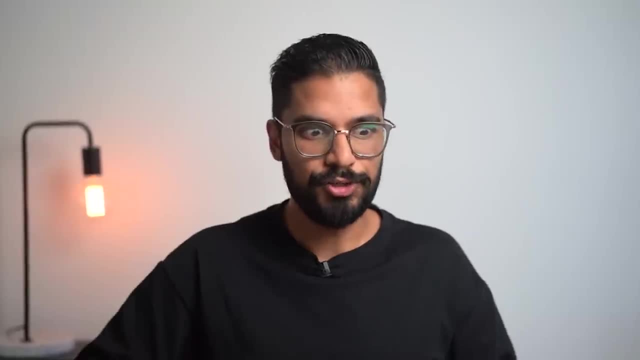 that I'm going to show you and with that, we're going to be able to determine what's going to happen over the next part of this cycle. Just like you have business cycles, economic cycles, you also have property cycles, believe it or not. And what's more is that you just don't have 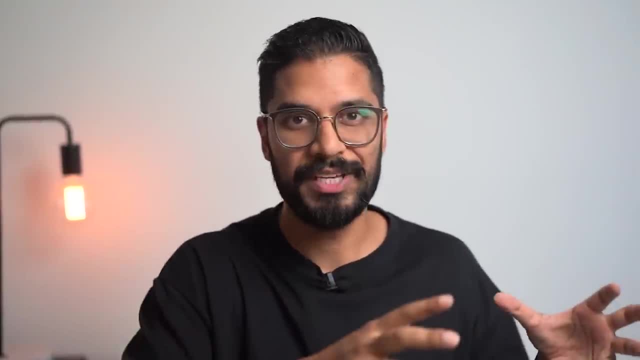 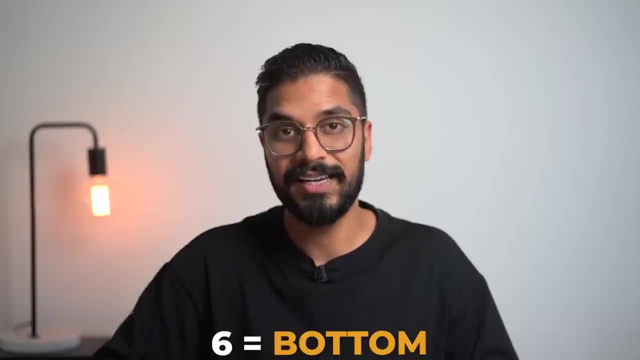 a cycle for all of Australia. In fact, there's different markets that have their own property cycle, and that's what people often refer to is like a property clock: If you're at 12,, you're basically at the peak of the market. If you're at 6,, you're at the bottom of the market. Anywhere between 6 and 9 o'clock is where you're starting to realize that upswing. It's essentially where we're trying to buy. If you're buying anything from 12 to 3, you're basically going to be in negative equity territory. That's pretty much like buying a property in an emotional market.